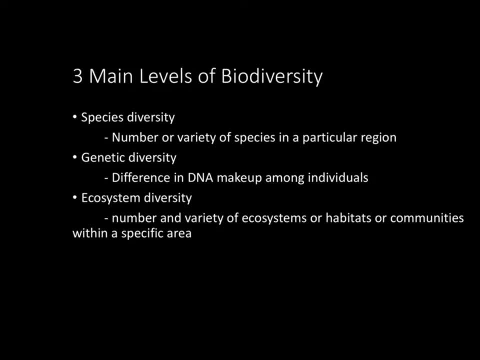 lines. it's important to note that biodiversity is really very hard to measure, And it's all of the measurements that we do have are going to be based on estimates, because how do you really measure biodiversity definitively? You can't, And then also, as it is hard to 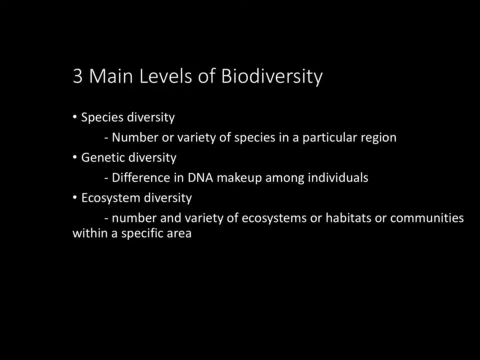 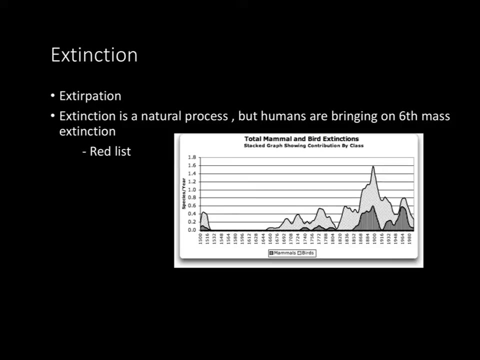 measure, it is unevenly distributed. Alright, so now let's take a look at extinction. Extinction basically means when a last member of a species dies and thus that species ceases to exist. Okay, a vocab word that you should know and not mix up with extinction is something known as extirpation And basically what that. 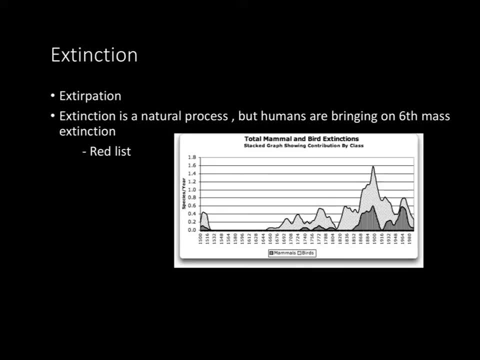 means is, let's say, a population in a certain area of a species dies. However, that doesn't mean the entire species itself is extinct because it still lives in other places. So take, for example, a fish living in a pond in Menlo Park. That fish does not live exclusively in that. 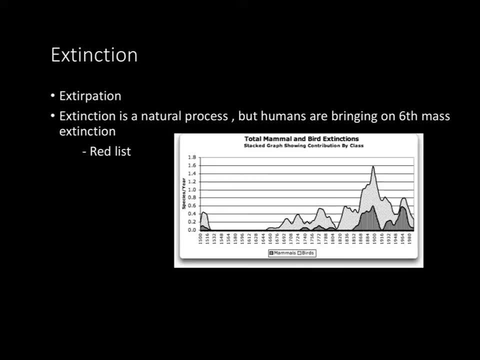 pond in Menlo Park. it lives all around the world. However, something happens to the environment in that specific pond and all the fish in that pond die. However, that does not mean that all the fish in the other ponds around the world die, and so that species isn't actually. 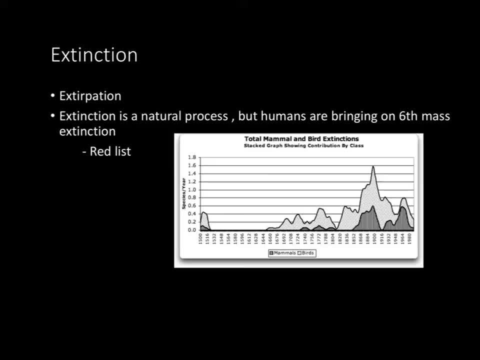 extinct. So that's a good example. Also, something to note about extinction is that extinction is a natural process. However, the problem is that we're speeding up this process much faster than it should occur. So extinction, as you can look down here at this graph, even though this is all human. 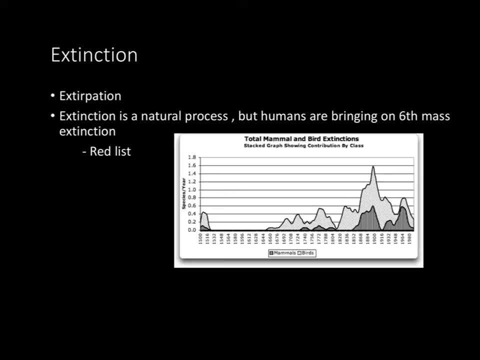 impact. extinction is a very natural process. Things are supposed to go extinct. However, with the human pollution and all of this and all of our building and habitat fragmentation, we're speeding up the process too quickly. We have something known as the red list, which 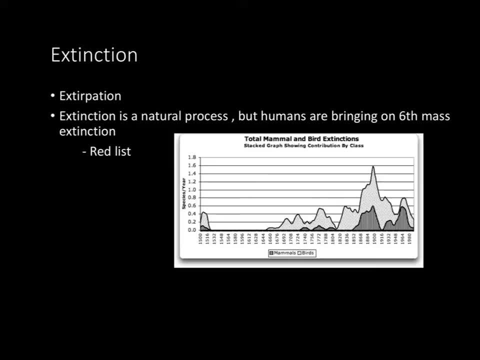 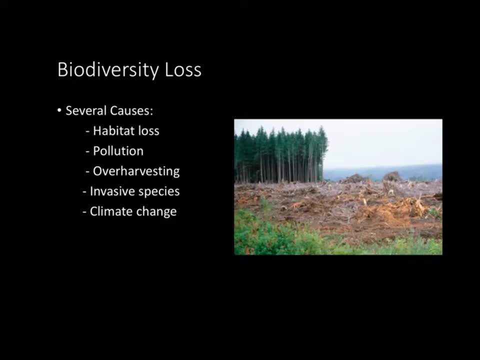 is basically a list of species that are rapidly heading towards extinction that we make sure to keep an eye out on as well. Alright, so now let's take a look at biodiversity loss. So there are going to be several main causes that we're going. 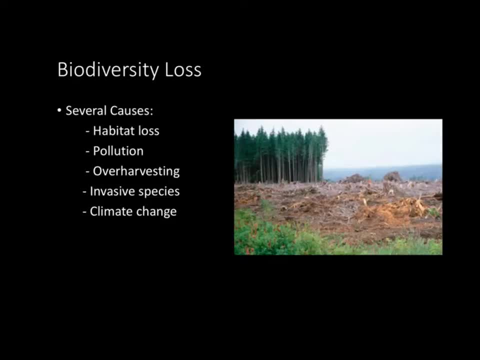 to investigate, the first of which is habitat. habitat loss, excuse me, which is the greatest cause? So when speaking about habitat loss, it can be directly outright habitat loss, so you can think about, like clear-cutting a forest, so that's direct habitat destruction, or it could be something such as habitat. 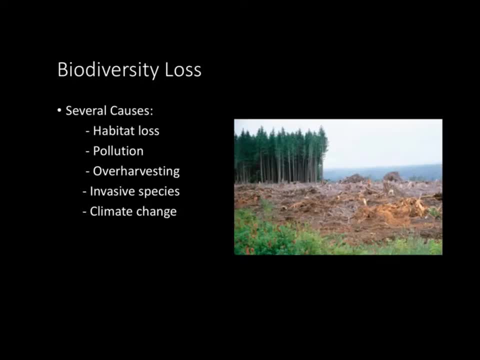 fragmentation. When looking at pollution, you could examine air pollution and water pollution and a couple other things as really main causes for losing biodiversity because, say for water pollution for example, eutrophication occurs, an entire pond ecosystem is now killed off and that biodiversity is gone. 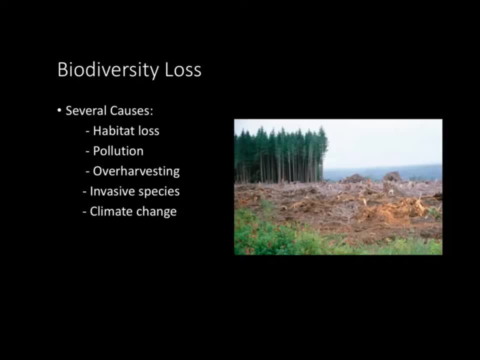 Over-harvesting. that's not referring to crops. in this case, that's going to refer to animal hunting, and so, basically, this is a problem when you're hunting large, long-living, case-select species such as like a tiger or something. 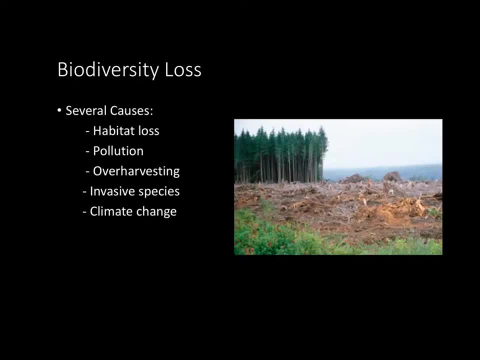 so that's going to be a problem when you're hunting large, long-living, case-select species such as like a tiger or something. it takes a longer time for them to reproduce and there are less of them. so if you over-harvest them and poach them, essentially, then they're not going to be. 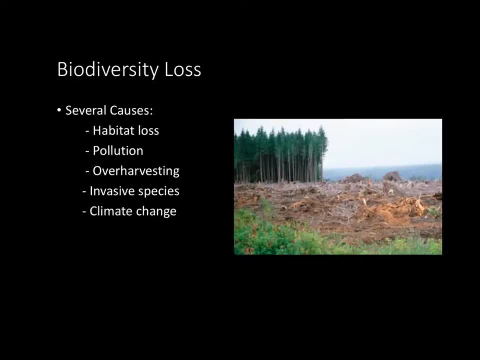 able to repopulate and that biodiversity goes down. Now, when you're looking at invasive species, you can see that as biodiversity loss because, say, like the cane toad, comes in and completely kills all of the native species and that kills off a lot of biodiversity that was there and now you only have this one cane toad. 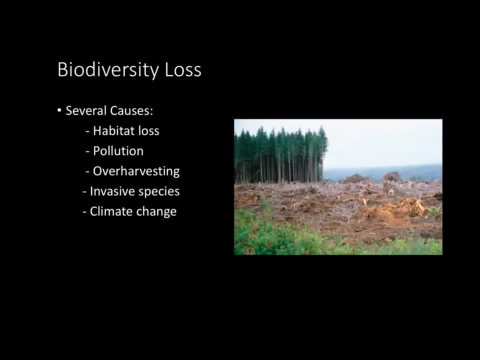 completely running everything and that's the only animal, So that's taking up biodiversity in that sense. If you look down here at climate change, climate change is a very general topic, but you could break that into say global warming and extreme weather conditions, and because of that, 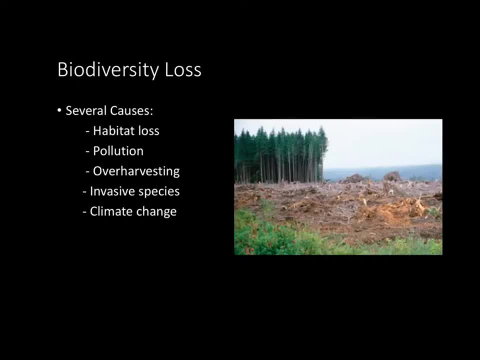 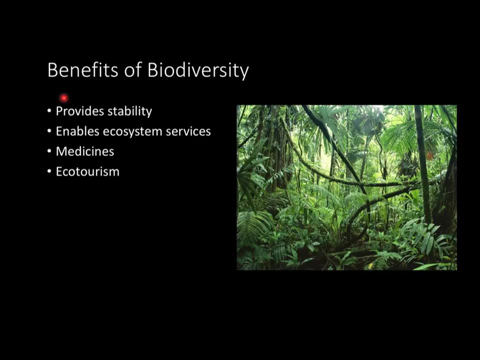 biodiversity is lost for a plethora of reasons. really, if you get a little more specific, All of these can relate to climate change as well. Alright, so now let's examine the benefits of biodiversity and why it's actually a good thing. So, first and 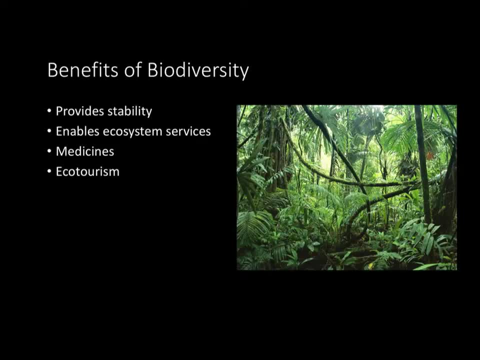 foremost, it provides stability. So the way I can explain this is: think about if you have a very, very intricate food web in a certain ecosystem, So say the rainforest, always a very biodiverse place. Say, a certain frog dies off and 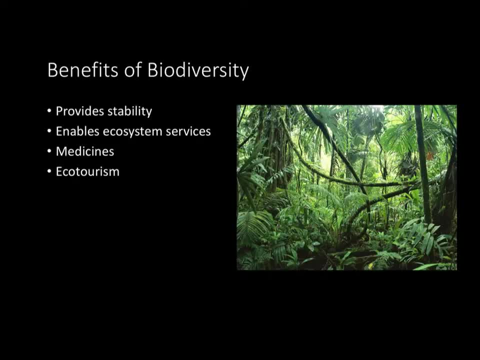 there's a lot of things dependent on that frog: What that frog eats. if it's not eating anymore, then the amount and the amount of individuals in the certain community is going to go way up and throw everything off, And it's also bad for the thing that eats the frog, because now they have nothing left to eat. However, if you have a lot of 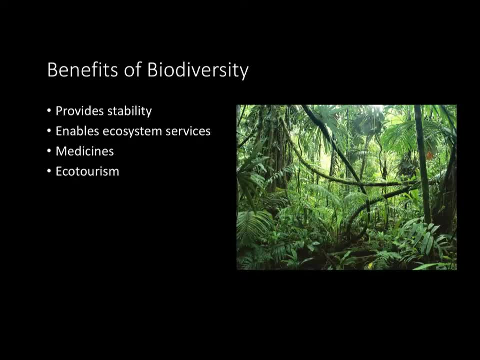 different frogs in the ecosystem. it's much more possible for things to adjust to eating The other frog and getting eaten by the other frog than it is if there are just no other frogs, So that's why it's always good to have a lot of different animals. Alright, so now let's talk about 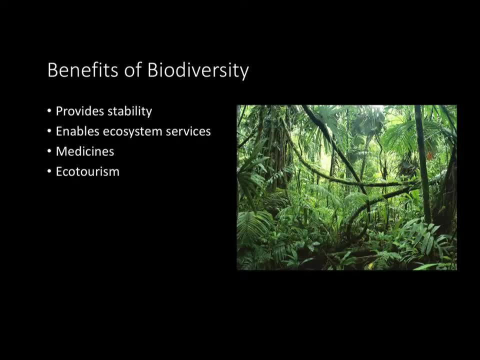 ecosystem services. So a refresher on those, that could be something such as pollination, the nitrogen cycle, a natural filtration cycle, really any of that. When you have a very biodiverse community that's very, very stable, that obviously helps those things happen. So bees are more ready, readily pollinating. 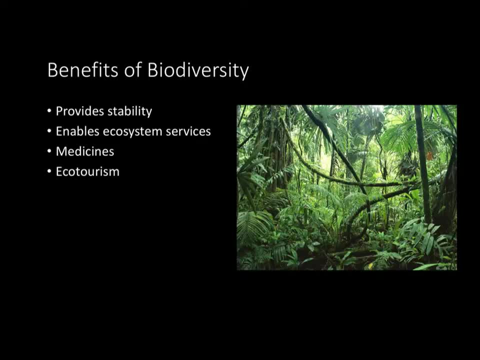 nitrogen cycles in full swing. It's very, very helpful Also. okay, so now let's take a look at medicines. So when looking at medicines, there are actually a ton of natural remedies that we use in our modern medicine that are only possible because of biodiversity. Okay, and now let's look at 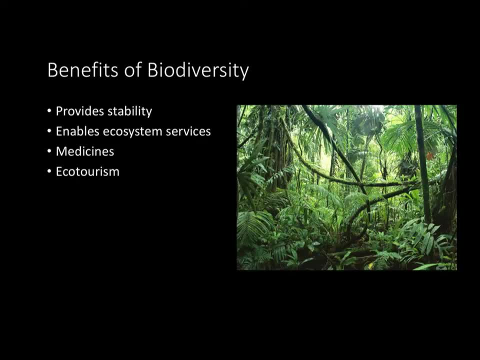 something known as ecotourism. So ecotourism is basically traveling to go see a natural site, And so that can generate a lot of money and actually be very helpful. And so ecotourism is really, really important because it generates a. 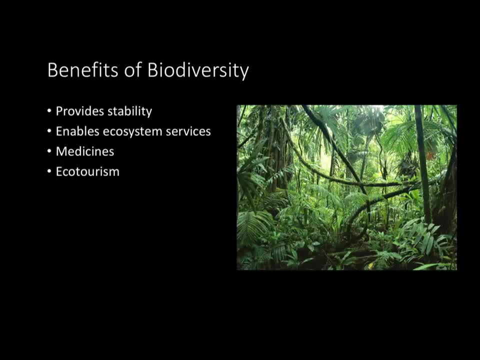 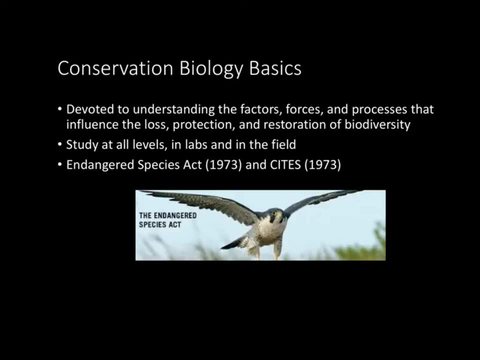 lot of revenue for places such as the rainforest, and without biodiversity it's not possible. Okay, let's take a look at conservation biology basics. So, basically, conservation biology is devoted to understanding the factors, forces and processes that influence the lost, protection and restoration of biodiversity. So within this there's a 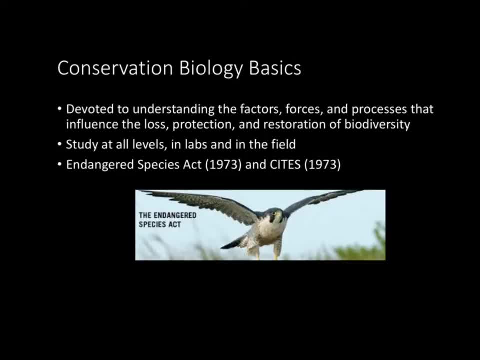 study at all levels, so in the labs and in the field. Basically, what that means is that conservation biologists are studying DNA and genes of certain animals in a lab while waiting. So if the—so as you can see- they're interested in. 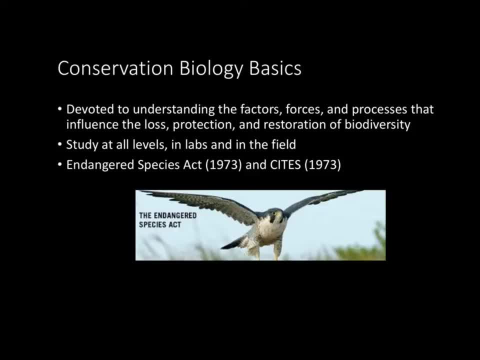 while they're also studying entire ecosystems out in the actual field and in nature, So it's a very wide-ranging, diverse field of study. There are two pretty important environmental laws you're going to want to have an understanding about that relate to conservation biology, and the biggest of those would be the Endangered Species Act. 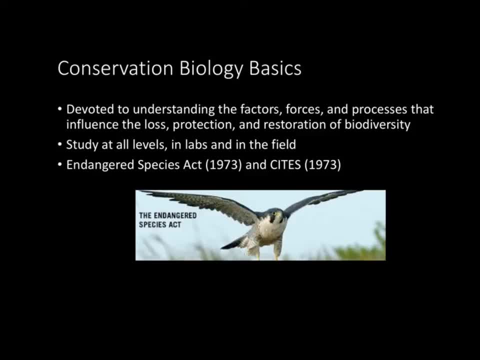 So that's something you're really going to want to have a very good understanding of for this course. And so basically, what the Endangered Species Act did was it was passed in 1973, and it basically says that it forbids anyone from harming an endangered species or their habitats. 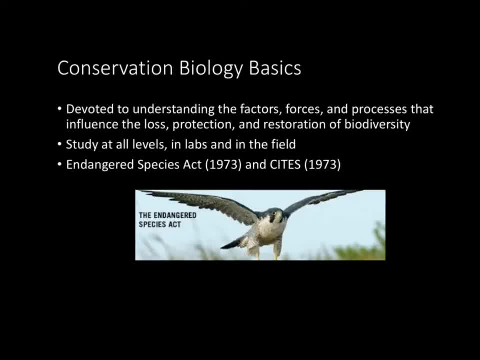 So say something was named an endangered species and put on the list. it's actually illegal for a corporation, or even an individual, to harm the habitat or the animal itself. Another important piece of environmental legislation is something known as CITES, or the proper long name, the Convention on International Trade in Endangered Species of Wildlife, Fauna and Flora. 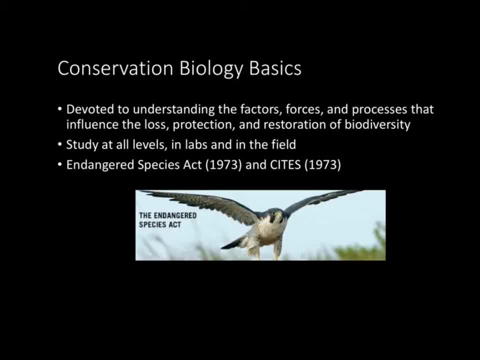 So it's a little easier to know the acronym. But basically what that says is that it doesn't allow any trading of endangered species. So basically, poaching- You can't poach an endangered tiger and sell body parts. That is now illegal and protected under the law. 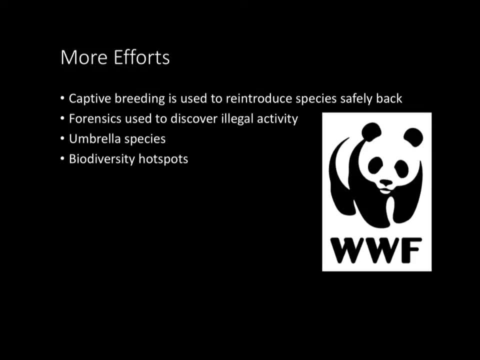 Okay, so more efforts. So there's something known as captive breeding, which is basically the captive breeding, so a human-run breeding of certain species within a controlled environment in which the animals are raised to a certain age and then reintroduced into nature. 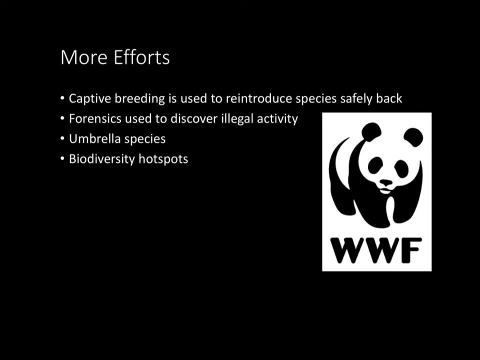 So this is basically used in order to ensure that certain species don't go extinct. So, say, there is an endangered bird, there's only a couple of them left. you want to make sure that they breed, You want to make sure that they reproduce and are reintroduced to nature properly, without being eaten or killed or anything. 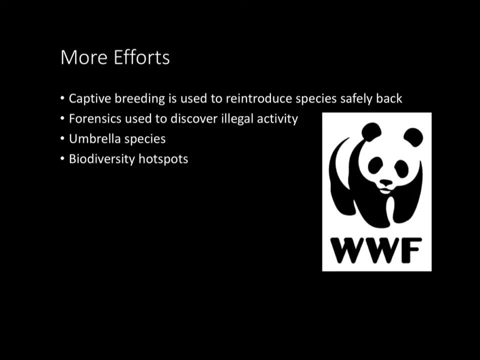 You could have them captively bred and then aged until they've reached maturity and then sent back into nature so they could prosper and the species could live on. So that's basically how that works. Okay, and then there's something known as forensics, which I'm sure you all know from CSI and cop shows. 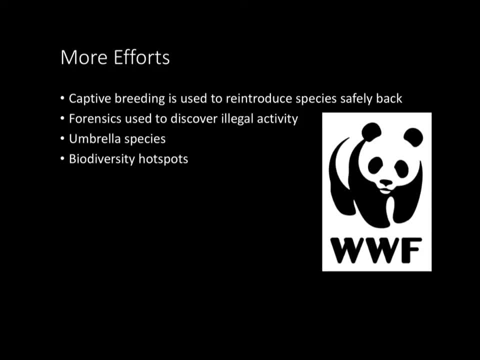 But basically it's the same kind of thing. So basically, forensics in this case refers to scientists discovering any illegal poaching and other types of activity in certain areas. They can use DNA and they can detect this and act accordingly. Okay, so now there's an interesting subject known as an umbrella species. 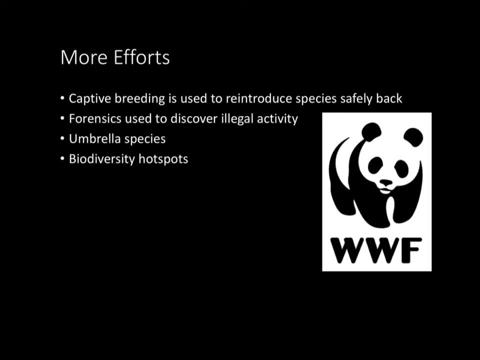 So you can refer down here to this panda bear which I'm sure we're all familiar with. He represents the World Wildlife Fund. So basically, an umbrella species is a flagship species. So by supporting this animal very publicly, an organization can ensure that the rest of 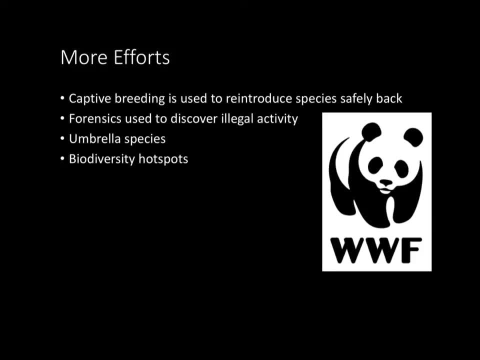 the ecosystem of that animal benefits. So say the World Wildlife Fund. in this case, takes the panda. By supporting a panda- which a panda bear everyone loves, who doesn't want to make sure a panda survives? By picking the panda, that ensures that the panda's entire ecosystem benefits from getting care. 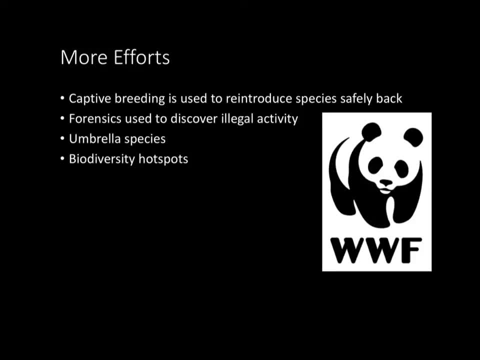 and getting money and making sure resources are there. So that's basically how an umbrella species works. Now, looking at a biodiversity hotspot, that's basically a way of prioritizing certain areas. So say, the most important areas would be sensitive areas with endemic species. that should receive the most attention. 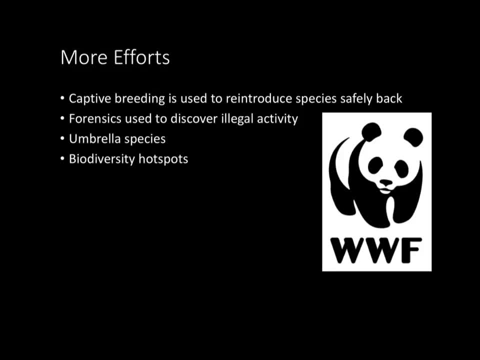 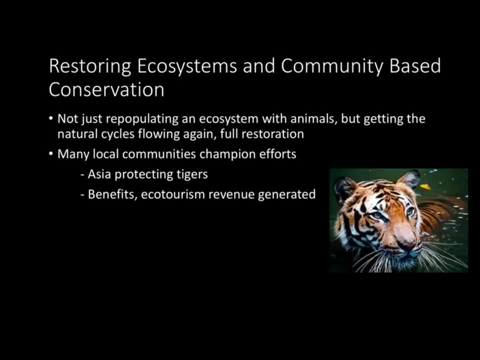 So that's basically just appropriating attention to where it's most needed. Okay, restoring ecosystems and community-based conservation. So restoring ecosystems, It's not just repopulating an ecosystem with animals, but it's actually getting the natural cycles flowing again. 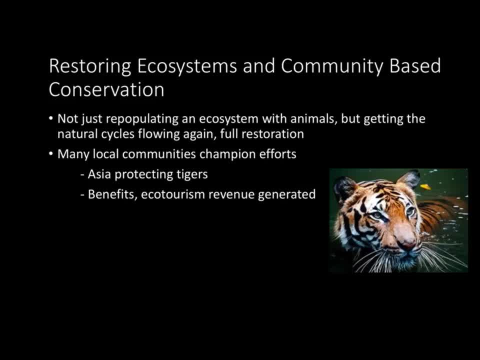 It's a forestoration. It's not just sending frogs back to a lake that has no more frogs. It's not just sending frogs back to a lake that has no more frogs, It's making sure that lake can actually support frogs for generations. 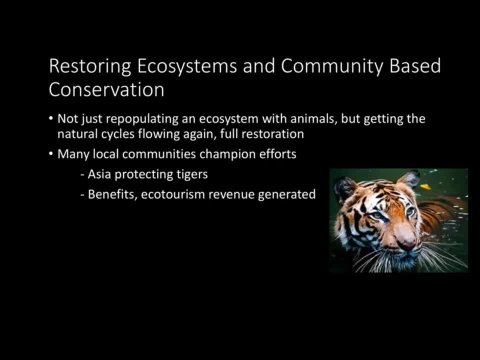 Okay, so now let's take a look at community-based conservation. So many local communities in certain countries are supporting efforts of conservation. So in Asia, a lot of different countries are protecting tigers. This is a good thing for them to do, because they do benefit directly. 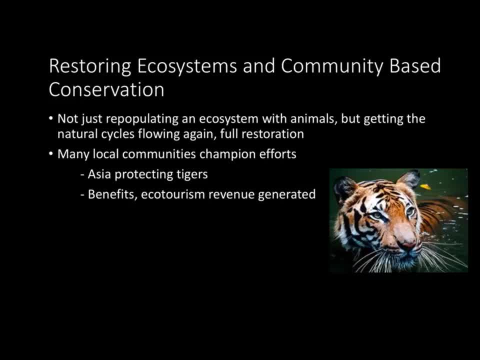 So say, a certain region in Asia has the capability and the natural environment to support these beautiful animals. If they make sure that these animals stay alive, then they're going to benefit from that ecotourism that we talked about earlier. People are going to come and want to see the tigers. 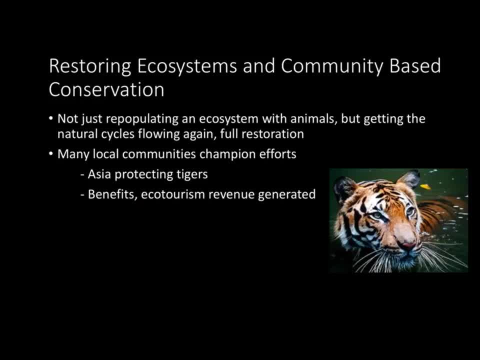 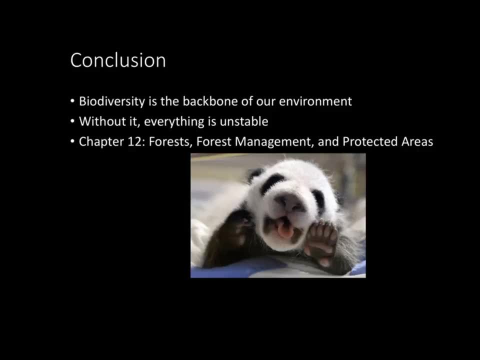 they're going to generate revenue for their town and everyone's going to benefit. Conclusion: Okay, so basically, biodiversity is the backbone of our environment. Without it, everything is unstable. In chapter 12, we're going to examine forests, forest management and protected areas. See you next time.